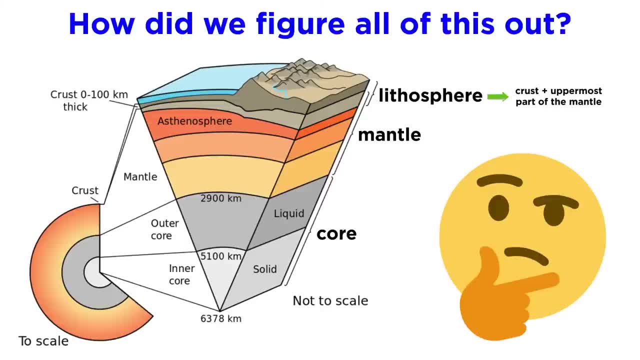 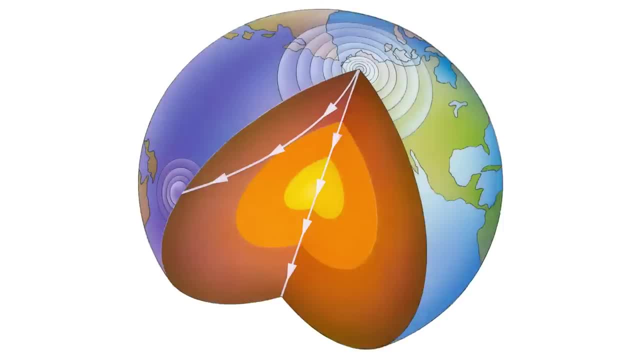 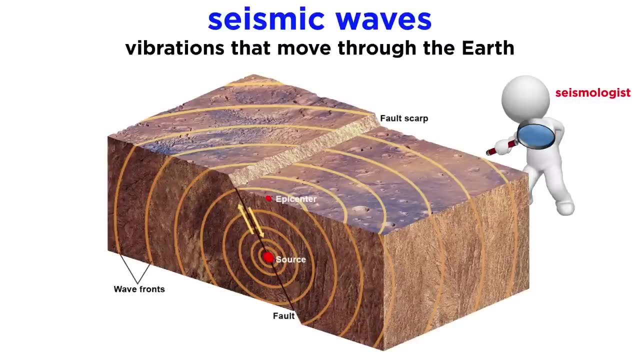 know anything about the physical properties of Earth's inner layers without actually visiting them? Geologists have come up with a clever way to answer this question: using seismic waves. Seismic waves are vibrations that rumble through the Earth. Seismologists, who are geologists that focus on seismic waves, study events like earthquakes, which release. 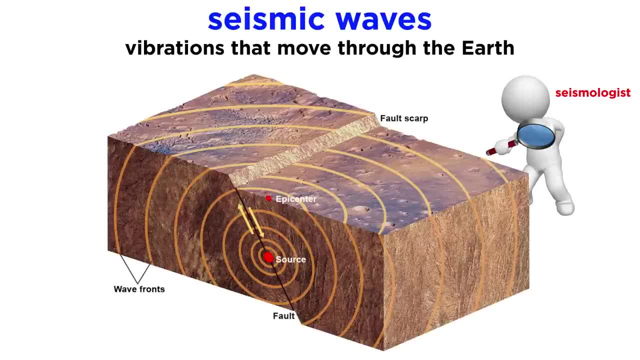 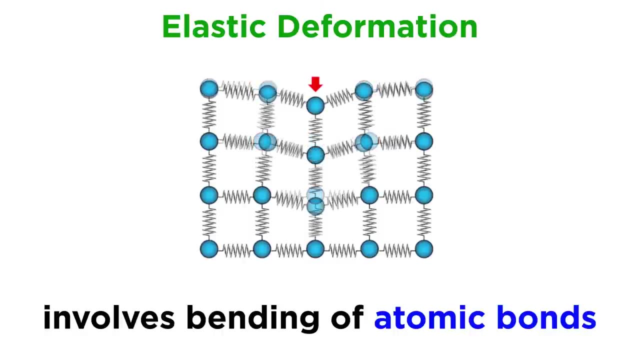 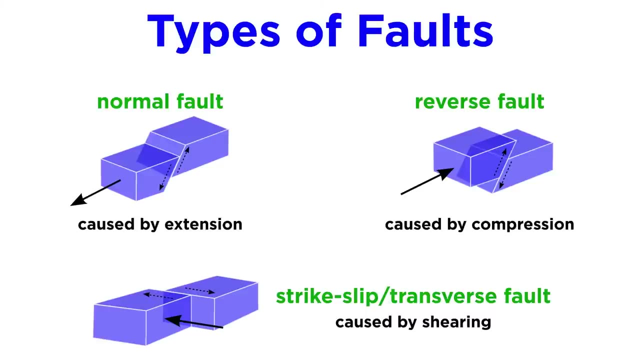 massive amounts of energy and produce seismic waves that ripple through Earth's layers. In an earlier tutorial on geologic structures, we discussed how rocks can undergo elastic deformation. When Earth's tectonic plates move past each other, they build up stress along their boundaries, which are massive faults. Over time, the stress 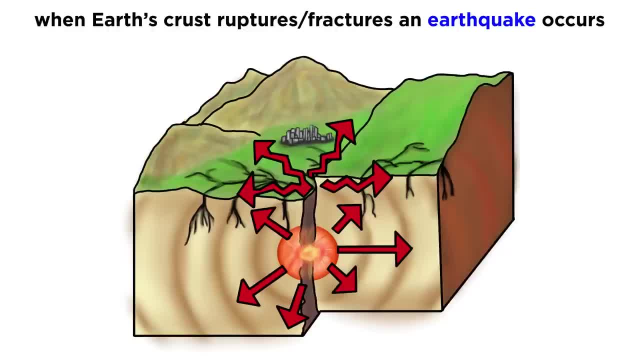 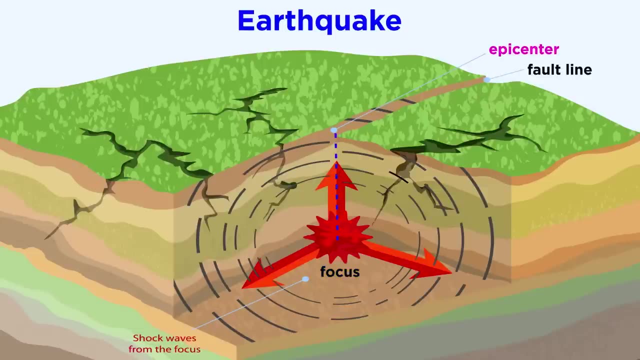 gradually increases until the crust can hold on no longer. The crust then ruptures and slides along the fault, releasing all the built-up stress in a burst of energy. The precise location within the crust that this burst occurs is called the focus. If you were to draw a straight line, 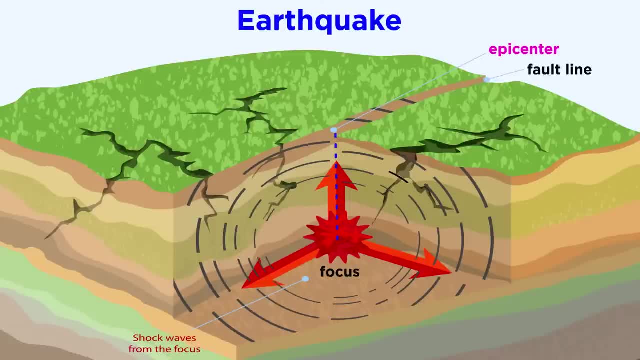 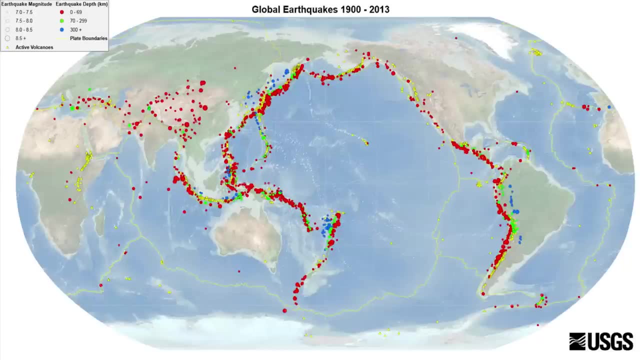 from the focus to the closest point on Earth's surface, you'd find the epicenter of the earthquake. By tracking the epicenters of earthquakes through time along a given fault zone, seismologists can predict the location of future earthquakes and provide early warnings. 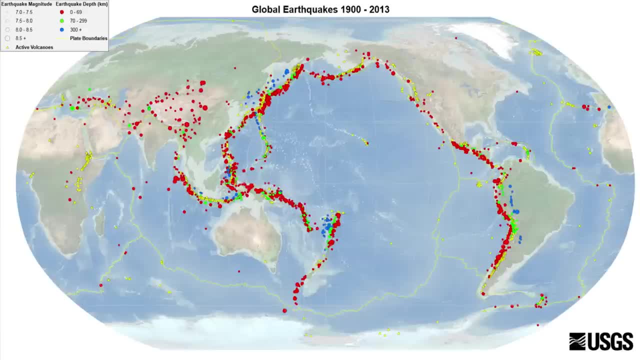 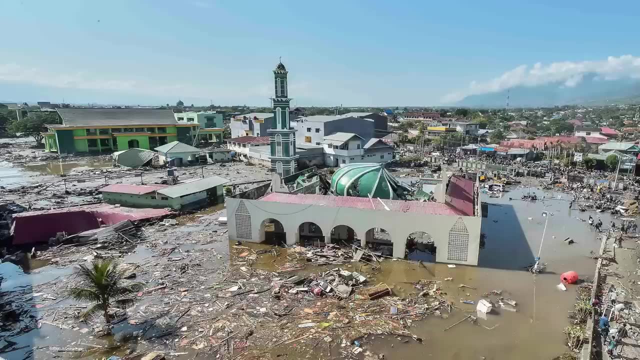 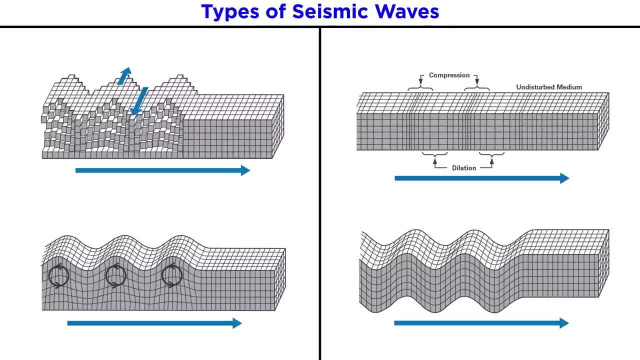 to citizens who live in earthquake-prone areas like California and Japan. When an area experiences a large earthquake, most of the stress is released and the fault needs time to build up more stress before another one can occur. Once an earthquake begins and energy is released at the 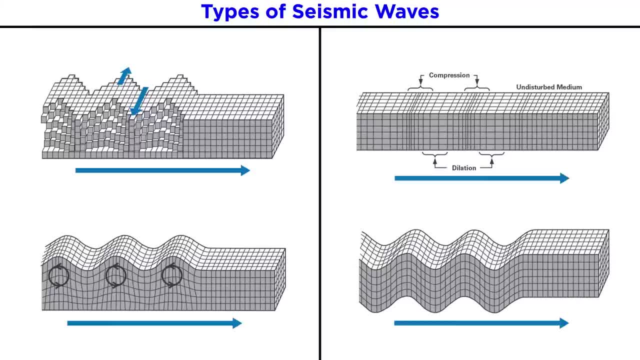 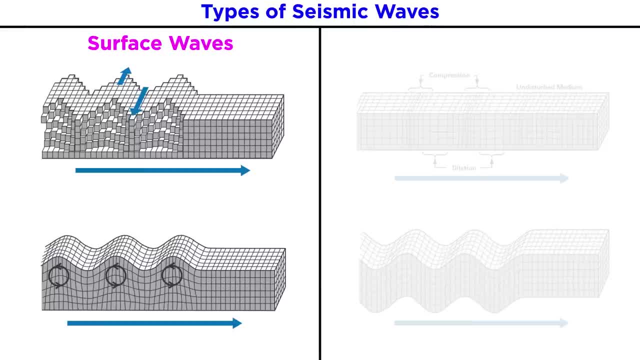 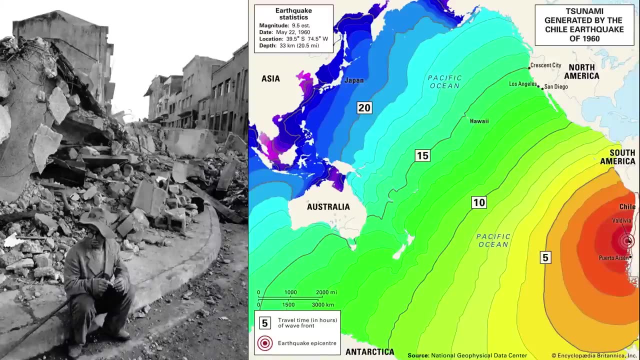 focus. several different types of seismic waves travel through the Earth's interior and along its surface. Surface waves are the seismic waves that travel through the shallow crust, potentially causing massive amounts of destruction. Surface waves from the 1960 Valdivia earthquake in Chile. 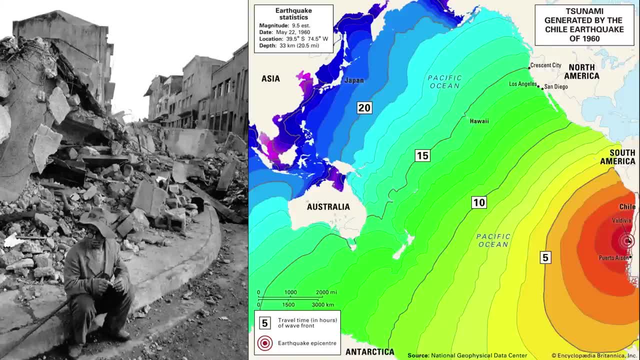 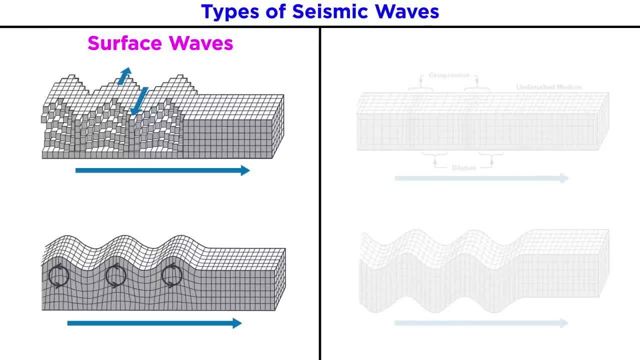 the most powerful earthquake ever recorded caused a tsunami that moved a ship almost a mile down the Valdivia River. There are two major earthquakes in the world. One is the earthquake in Chile, the second is the earthquake in Chile and the third is the earthquake in Chile. 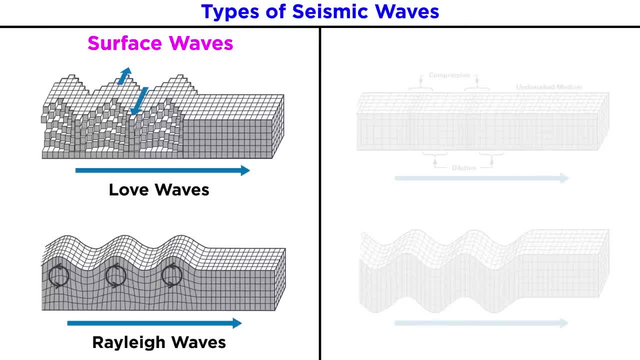 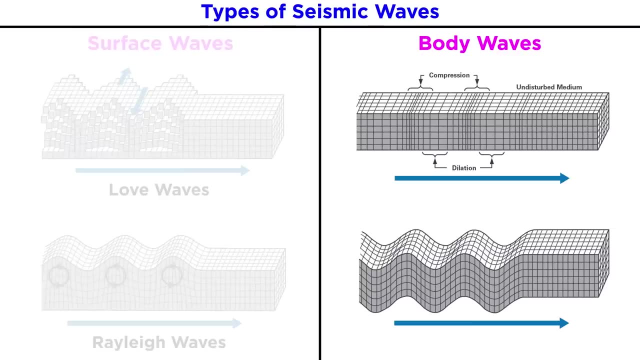 the three main types of surface waves: Love waves and Rayleigh waves. Love waves wiggle through Earth's surface side to side, like a snake slithering along the ground. Rayleigh waves roll along the surface, as do waves in the ocean, The seismic waves that travel through the Earth's 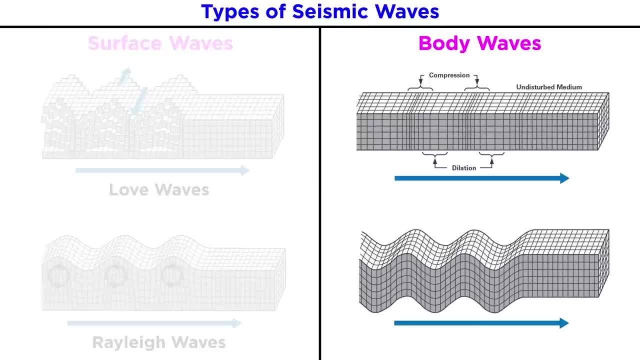 interior are called body waves. Body waves come in two types: S-waves and P-waves. P-waves are compressional like sound waves and wave motions that are not compressional like sound waves, and wave motion is parallel to propagation. S waves are shear waves, with wave motion being 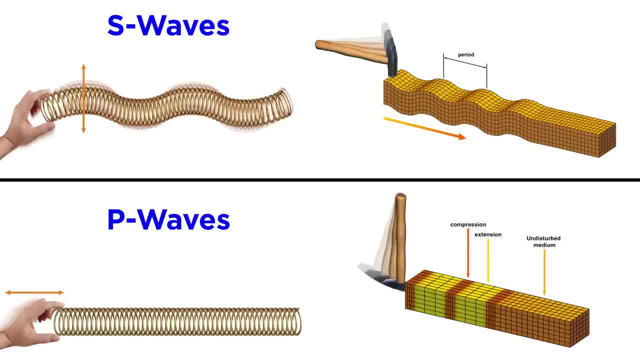 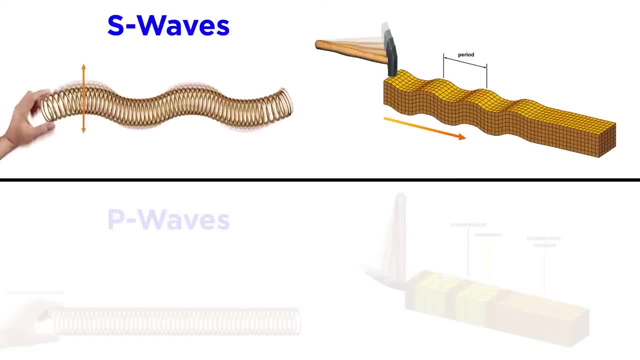 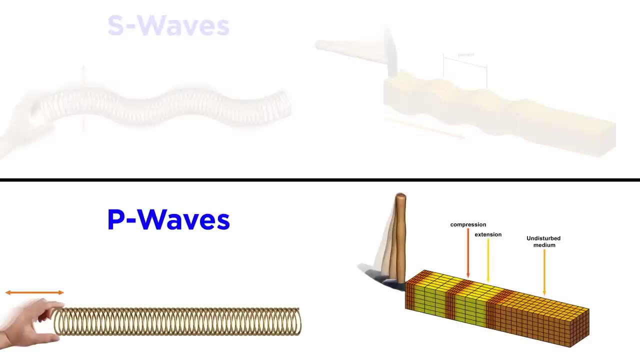 perpendicular to propagation. A slinky is often used to represent P and S waves. If a stretched out slinky is waved up and down at one end, that S wave will move along the slinky to the other end. If the same slinky is nudged forward or backward, a P wave will form. 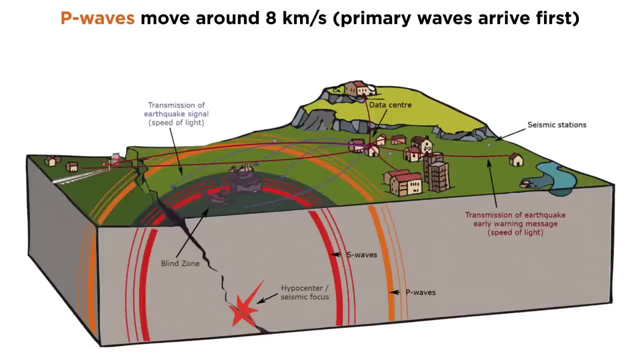 P waves are the fastest seismic wave and have velocities of around 8 kilometers per second, which is why P stands for primary, as these waves arrive first. S waves are a bit slower, with velocities of around 3.5 kilometers per second, which is why S stands for secondary. 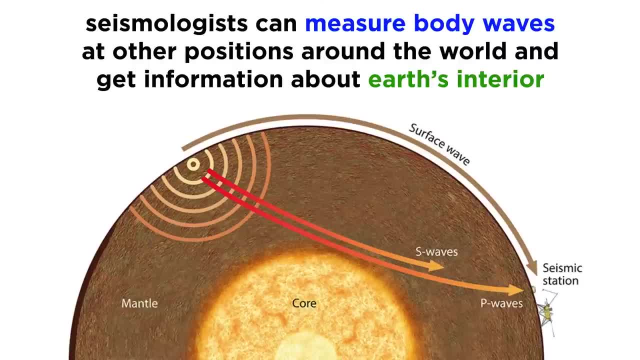 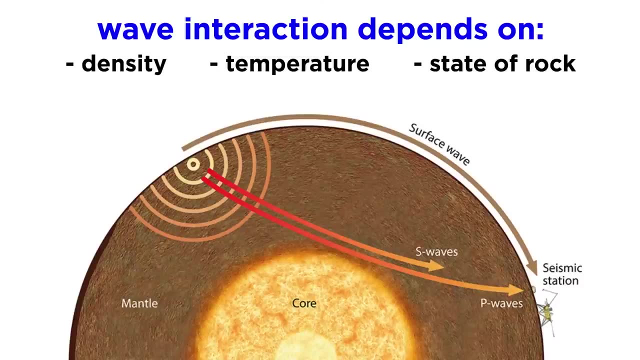 since they arrive. second, By measuring the types of body waves that travel through the planet's interior during earthquakes and their velocities, seismologists have built up a sort of echogram of Earth. The waves interact with Earth differently depending on the density, temperature and state of the rocks they travel through. When a propagating 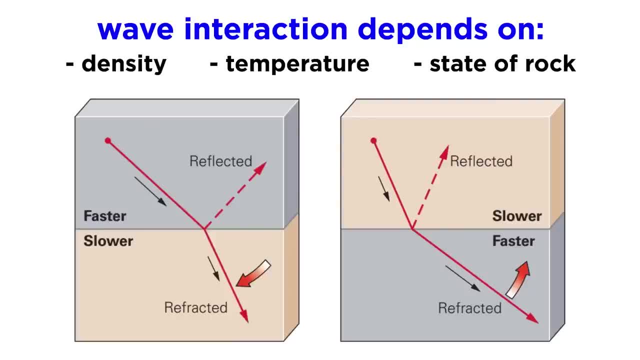 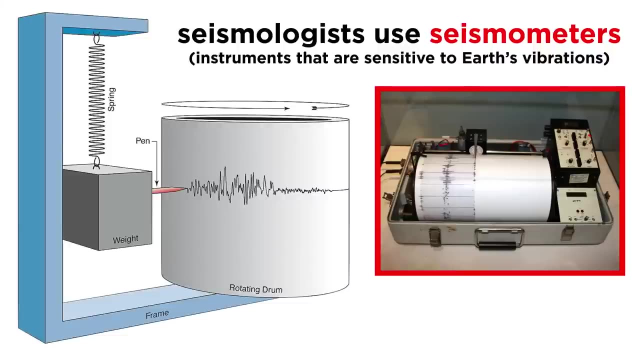 wave encounters a change in these properties- say, for example, at the boundary between the crust and the mantle, part of the wave will be reflected back towards the focus, with the remainder refracting into the new layer as the wave's velocity changes. Seismologists use instruments. 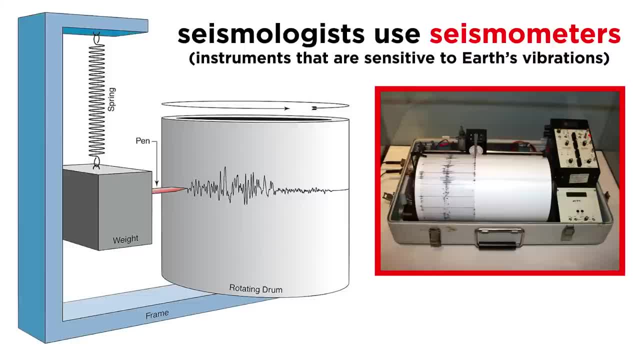 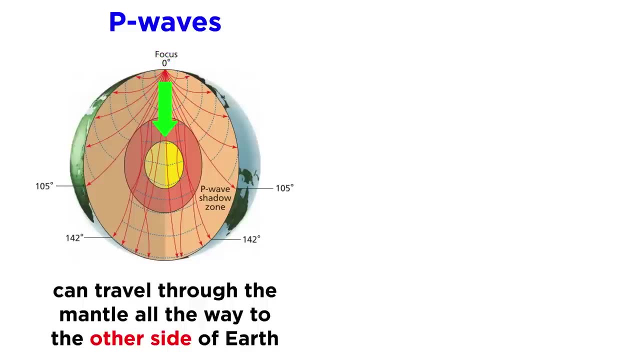 sensitive to Earth's vibrations, called seismometers to measure the S and P waves from earthquakes, as well as man-made sources like nuclear explosions and mining activity. P waves are able to travel from the focus in the crust through the solid mantle onwards through the 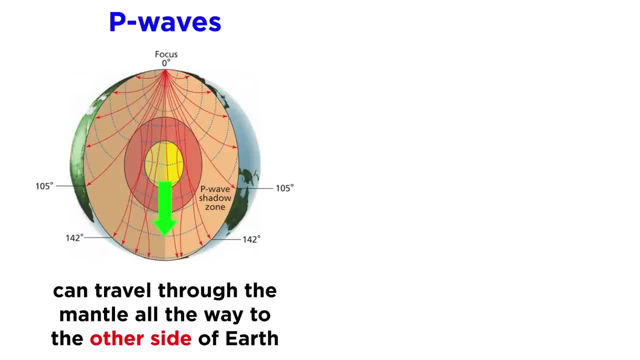 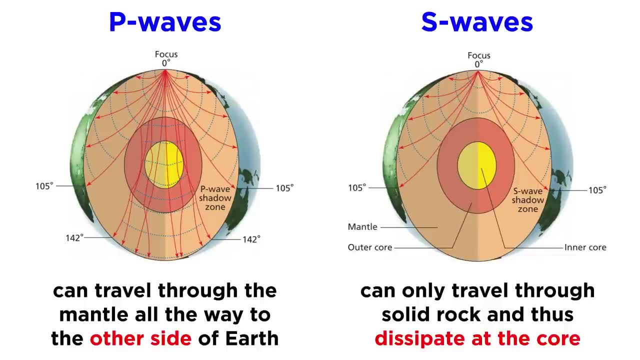 liquid and solid core and then back through the mantle to the opposite side of Earth. S waves, however, can only travel through solid rock. Since S waves can only travel through solid rock, these waves are dissipated at the outer core, A large area of Earth opposite the focus lacks. 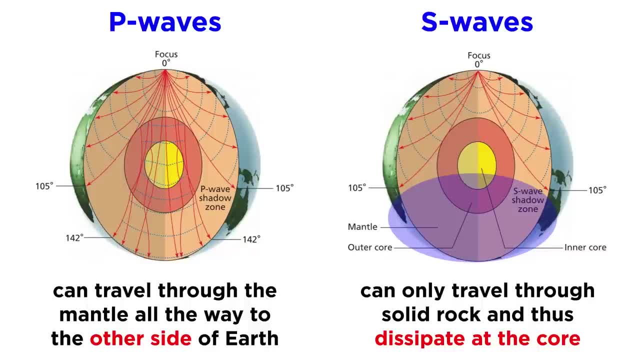 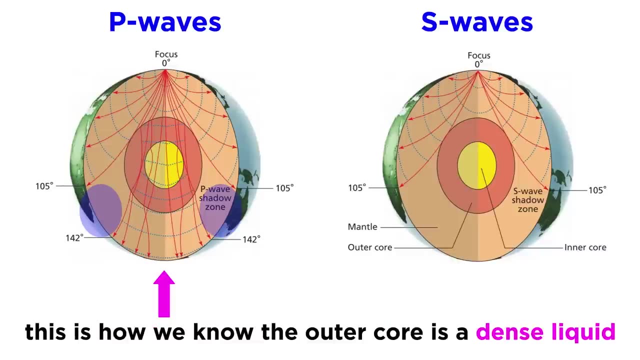 transmitted S waves. This is called the S wave shadow zone. There is also a P wave shadow zone caused by the refraction of P waves that occurs at the core-mantle boundary due to the dramatic increase in density that occurs there. This is how we know that the 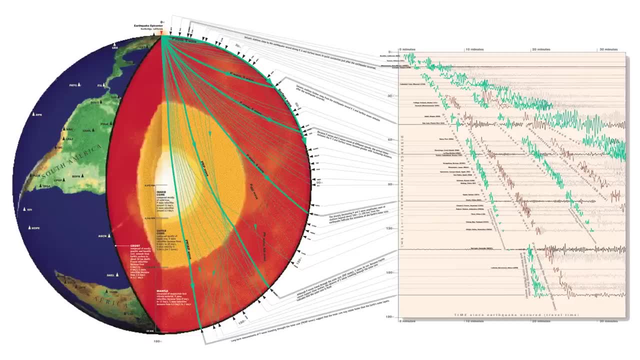 outer core is in a dense liquid state. With an increasing network of seismometers all over the planet, seismologists have been able to use seismic waves to resolve Earth's layers with increasing accuracy, especially the many sub-layers of the mantle. Speaking of the mantle, both P and 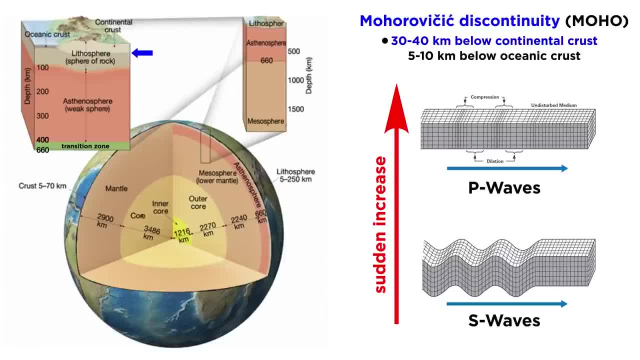 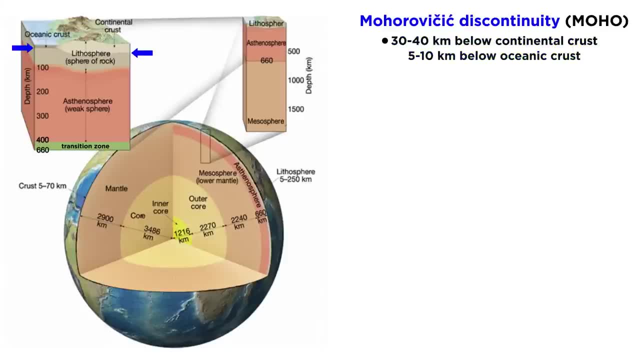 S wave velocities suddenly increase at around 30 to 40 kilometers below continental crust and 5 to 10 kilometers beneath oceanic crust. This layer, the Mohorovicic discontinuity, or MOHO, marks a sudden increase in density and is the boundary between the crust and denser mantle. Then, at 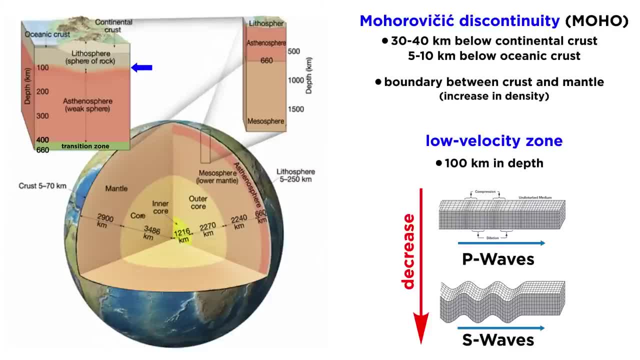 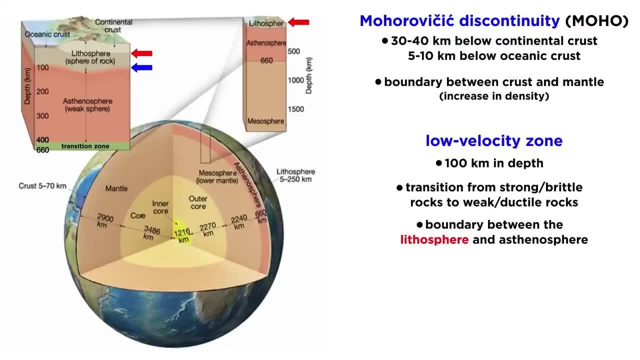 around 100 kilometers of depth there is a large decrease in body wave velocity, which is called the low velocity zone. This marks the transition from strong brittle rocks to weak ductile rocks. The brittle layer above the low velocity zone is called the lithosphere. 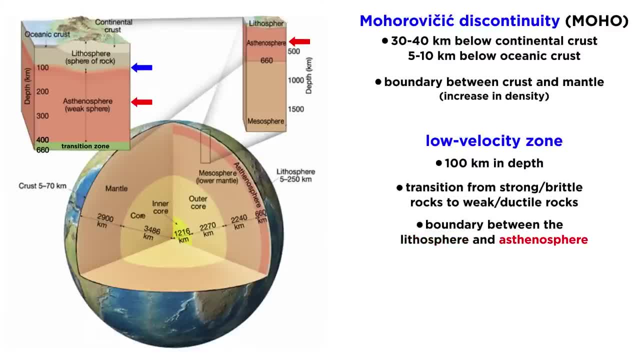 and it contains the crust and uppermost mantle. The ductile layer below is called the asthenosphere, and this is where the mantle is able to flow, marking the boundary between brittle and plastic deformation. The low velocity zone is unusual because seismic velocities usually increase with depth Its existence. 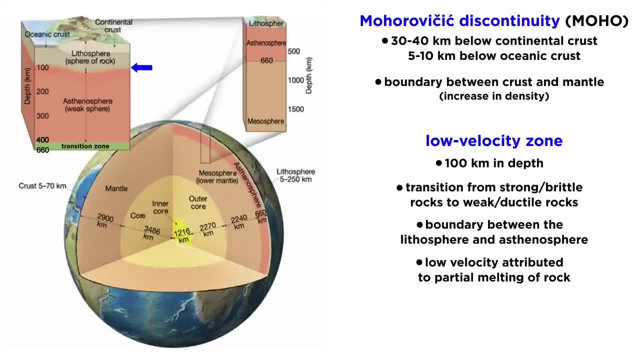 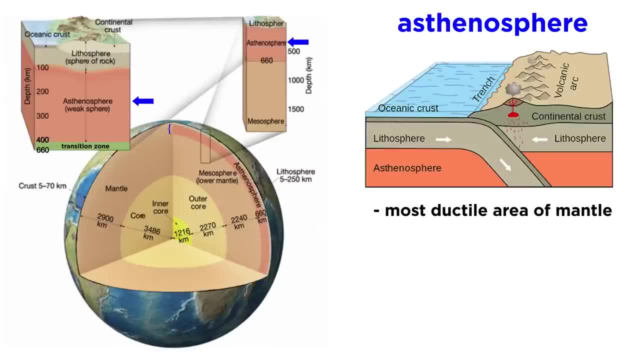 is attributed to 1 to 5 percent partial melting of mantle rock. The asthenosphere is the most ductile area of the mantle and extends down to 350 kilometers below the surface Continent-sized slabs of the lithosphere, which again are called tectonic. 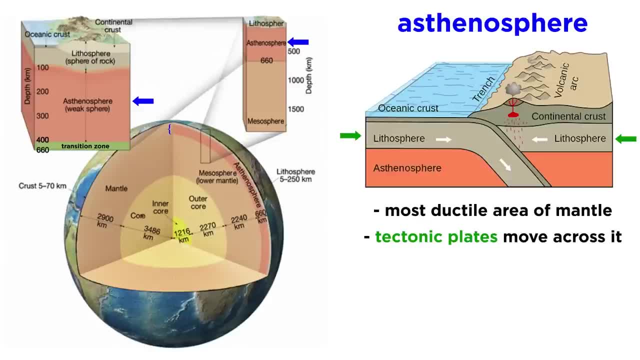 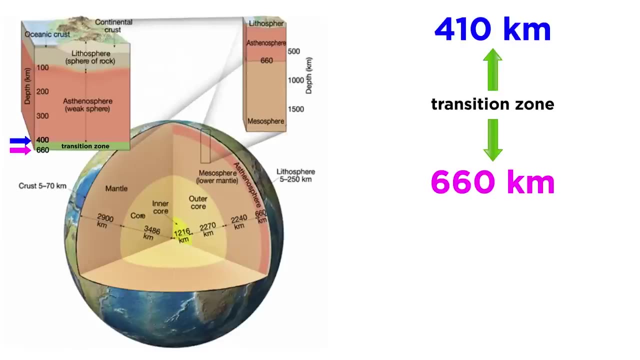 plates move along the top of the asthenosphere. Earthquakes and volcanic activity typically occur at the boundaries of tectonic plates, where they collide or slide past each other. The lower asthenosphere contains two additional abrupt increases in seismic velocities. 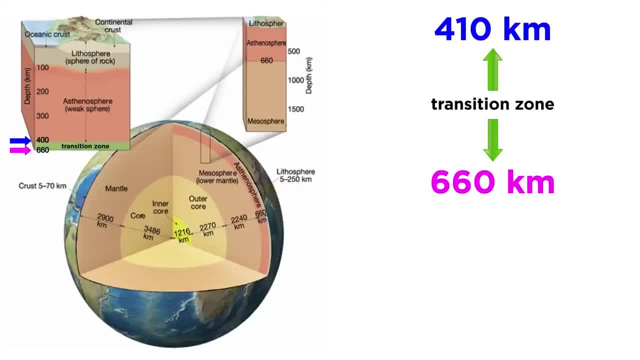 one at 410 and another at 660 kilometers. The area in between these two discontinuities is called the transition zone Here. olivine, the dominant mineral in the mantle, changes crystalline structure, becoming more dense to accommodate extreme pressures. 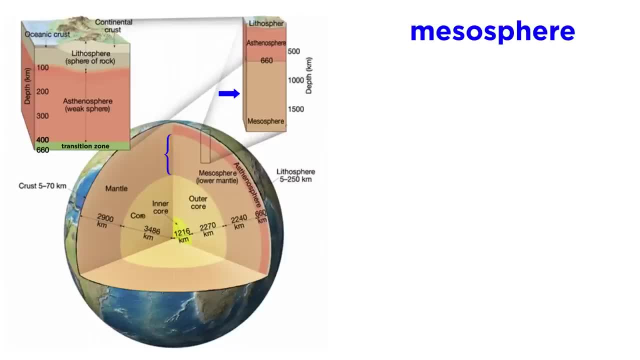 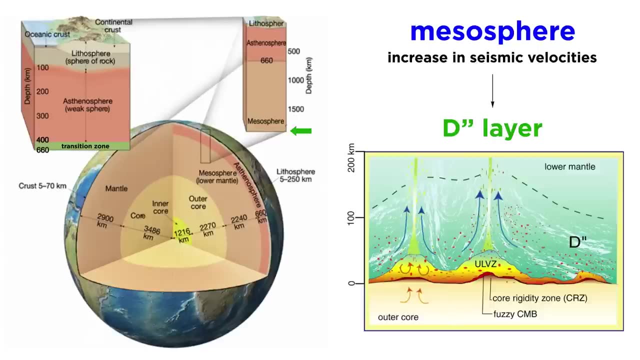 Below the 660 kilometer boundary is the lower mantle, or mesosphere, which is marked by a very steady increase in seismic velocities. At the bottom of the mantle lies the d-double prime layer, which is identified by an area of anomalously low and variable seismic velocities. 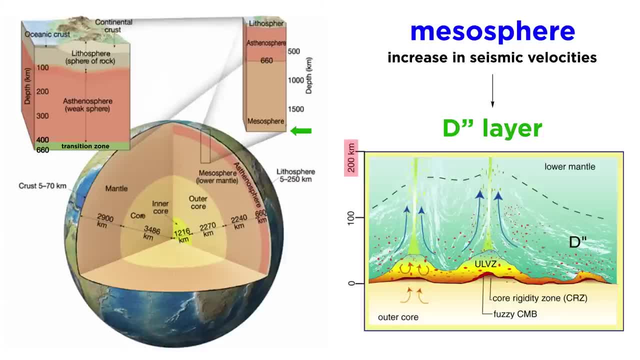 The d-double prime layer is about 200 kilometers thick and is probably heterogeneous in composition. At the very base of d-double prime, right at the core-mantle boundary, exists an ultra-low velocity zone, The name of this thin, laterally discontinuous layer, 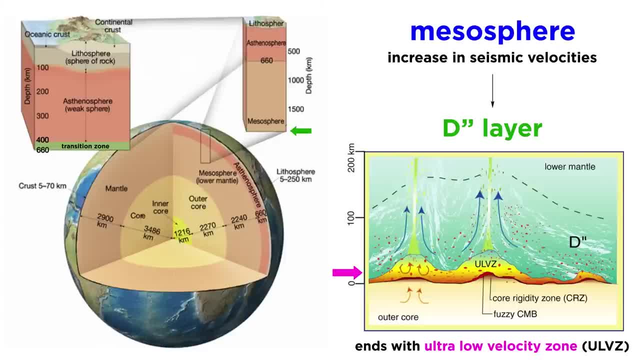 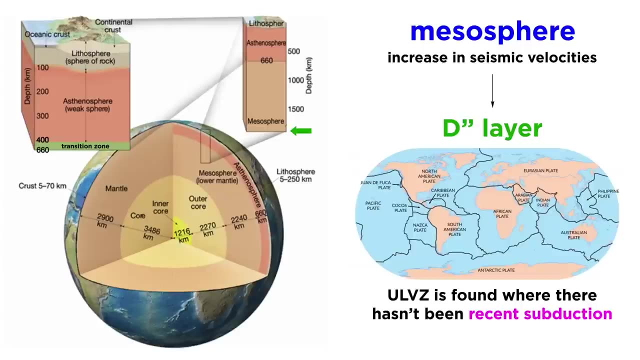 speaks for itself, as it is characterized by extremely low seismic velocities compared to surrounding mantle. The exact nature of this layer is a topic of much debate. It may represent an area of partial melting due to increased heat flux from the core. Ultra-low velocity zones only seem to exist in areas where there hasn't been recent subduction. 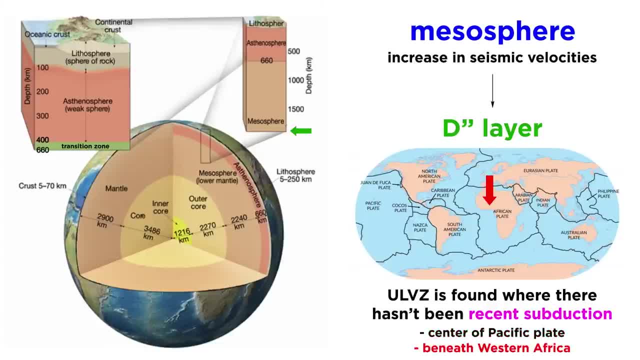 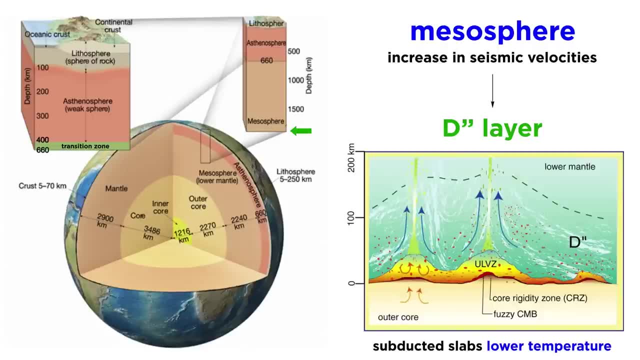 One exists beneath the center of the Pacific plate, the other beneath Western Africa. If subducted slabs indeed end up sinking to d-double prime, they will have the effect of lowering the temperature in that area, potentially influencing convection patterns in the outer core. 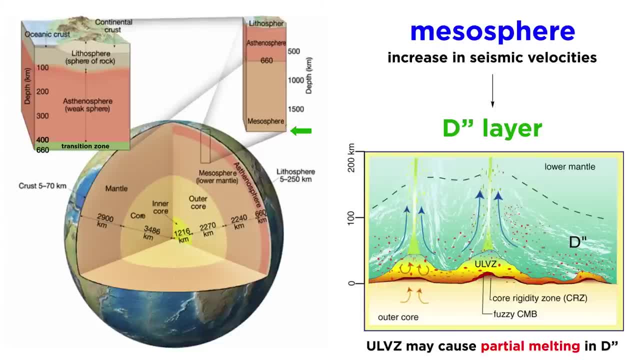 as well as core-mantle heat flux. Therefore, ultra-low velocity zones may represent areas beneath the hot, upward-convecting outer core, which causes partial melting of the d-double prime layer above, potentially initiating large mantle plumes called superplumes. 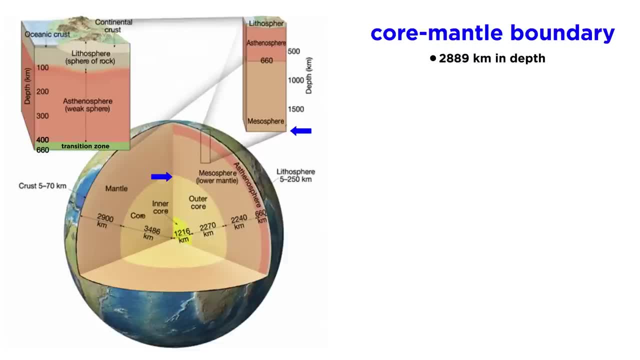 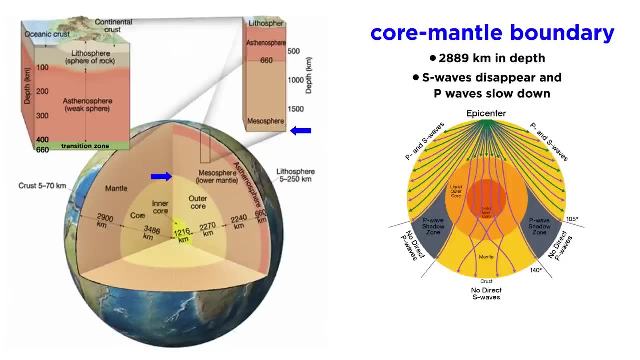 At a depth of 2,889 kilometers is the core-mantle boundary, which is defined by the disappearance of S-waves and a slowing of P-waves due to the outer core being in the liquid state, P-wave velocity steadily increases with depth in.